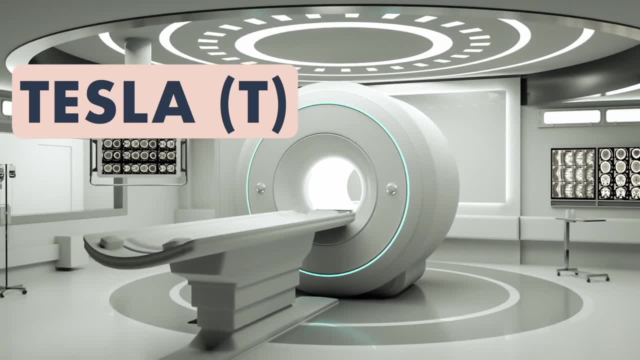 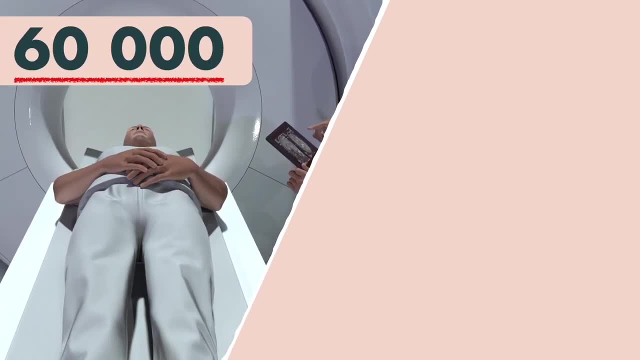 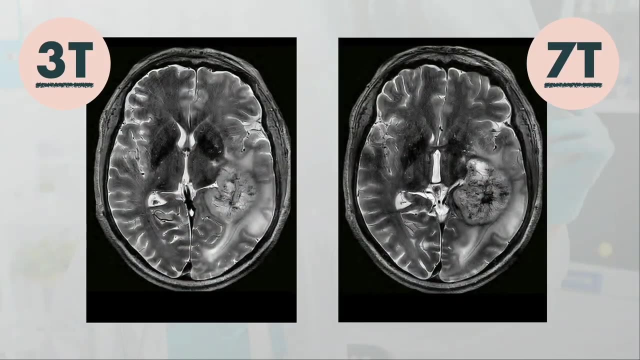 a unit called Tesla. Most MRI scanners used in hospitals are 1.5 or 3 Tesla. Putting that into perspective, a 3 Tesla MRI scanner is around 60,000 times stronger than the Earth's magnetic field. The stronger the magnetic field, the more detailed the images become, Which means the 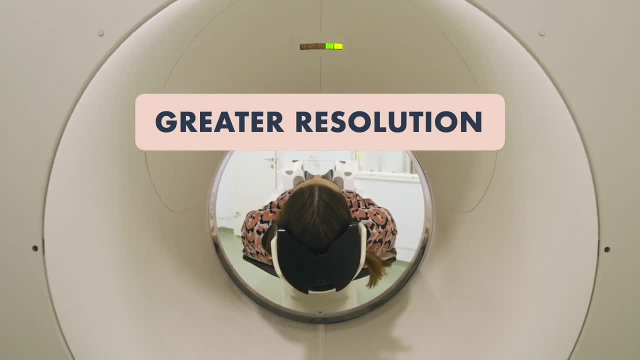 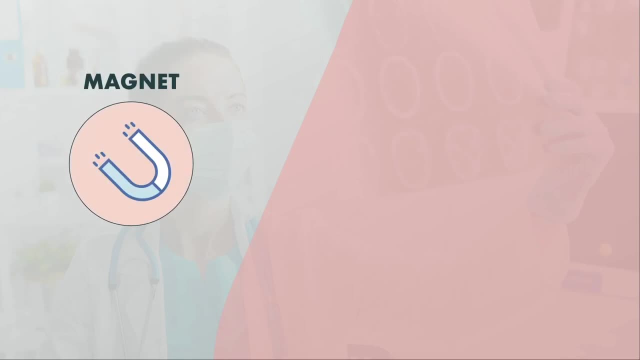 body can be imaged either at a greater resolution or at the same resolution, but faster. MRI uses magnetic fields and radio waves to measure how much water there is in different tissues of the body, and then uses this information to generate a detailed image. The images are so detailed because our bodies are pretty much entirely made of water. Our 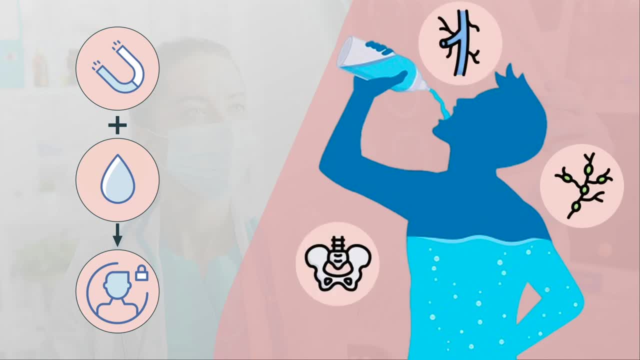 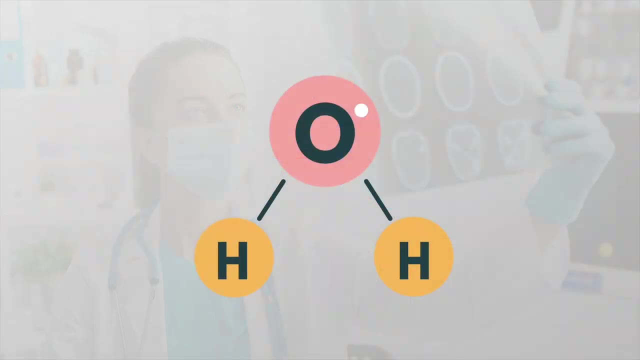 lymph nodes, our blood vessels and even our bones are soaked with water molecules. A water molecule is made up of two hydrogen atoms and one oxygen atom. The hydrogen atoms are the part that makes water interesting for MRI. If we look at hydrogen in more detail, 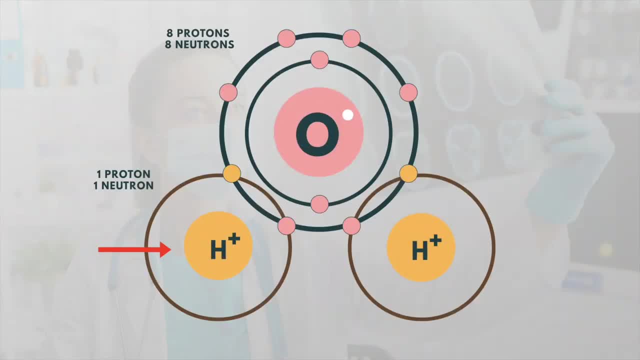 we see that it has a central nucleus containing a single positive charge called a proton. The hydrogen atom is the part that makes water interesting for MRI. If we look at hydrogen in more detail, we see that it has a central nucleus containing a single positive charge. 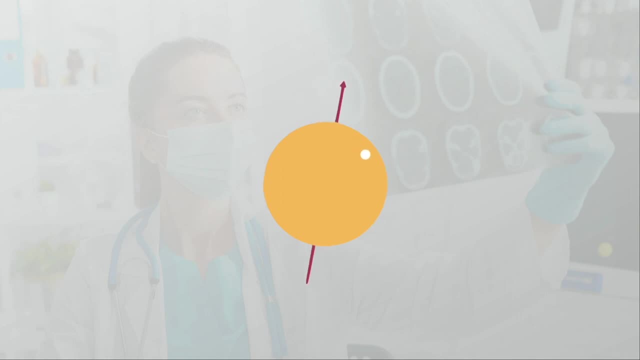 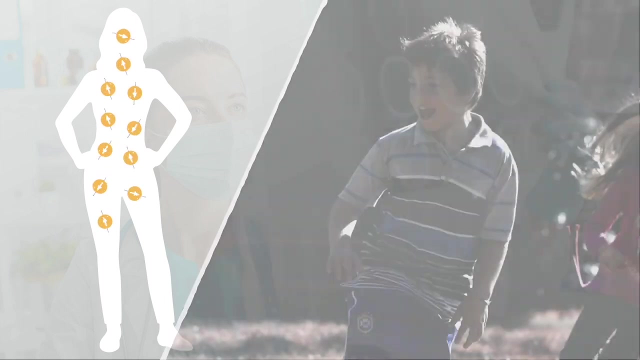 called a proton. Each spinning hydrogen proton is like a tiny magnet that spins around on its own axis. This spinning motion is known as precession. Under normal conditions, all the billions of hydrogen protons are in random positions spinning on their axis. Think of it as a group. 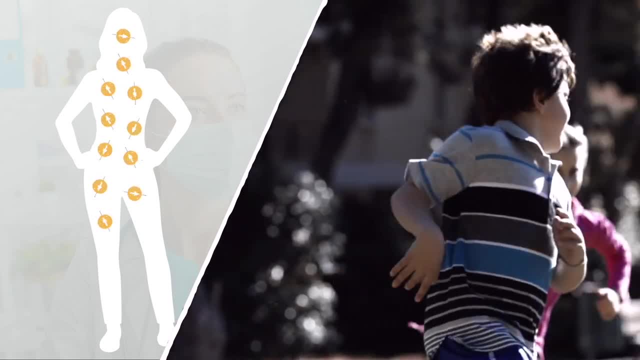 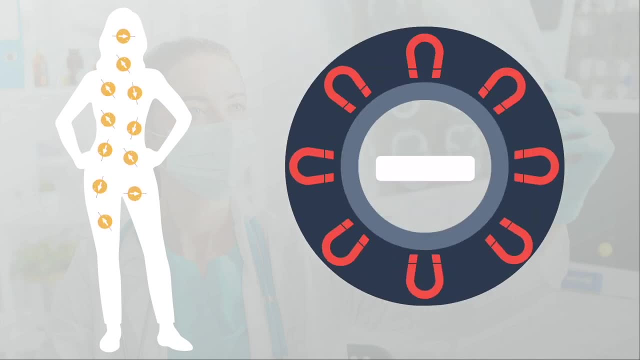 of children on a playground, running around with no sense of order. However, this randomness changes when we place a human body into a very strong magnetic field. Just like the north and south poles of a compass tend to align with the magnetic poles of the earth, in the presence of a strong magnetic field, each proton in water twists its orientation. 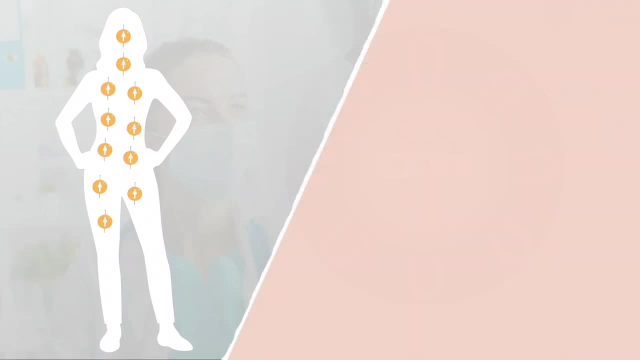 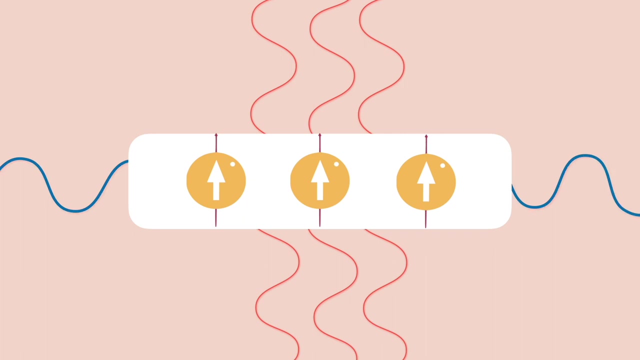 so that it aligns with the field. Now think of those same children with no order and how each one will line up when the teacher calls. But while the magnetic field makes all the protons want to line up, the MRI machine intentionally disrupts this field by sending a brief pulse of an additional, weaker electromagnetic field.